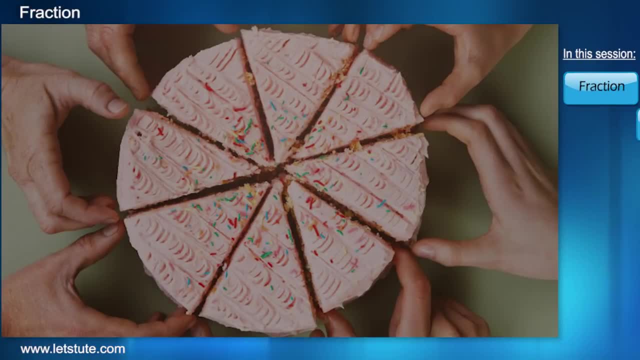 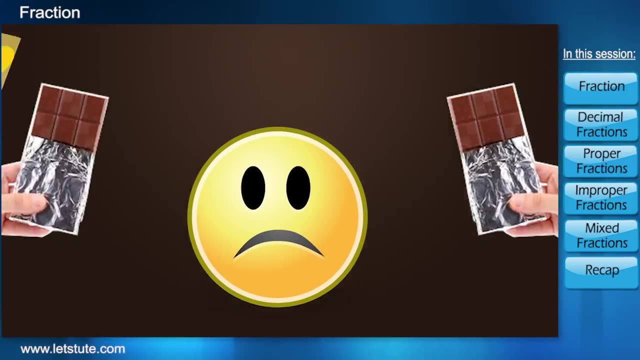 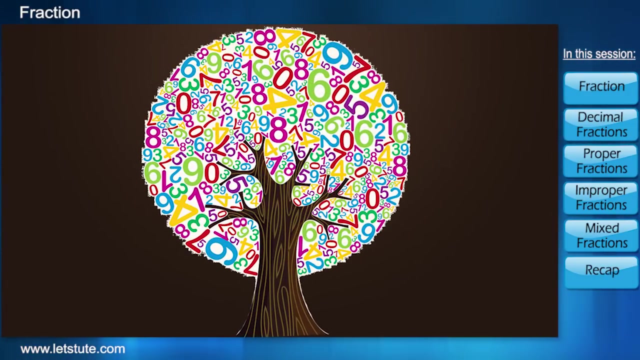 Sharing is caring, But when it comes to chocolate, no one likes to share them, isn't it? When you share something or divide something, there is a lot of mathematics behind it. So, without wasting any time, let's start this session with you and some of your friends. 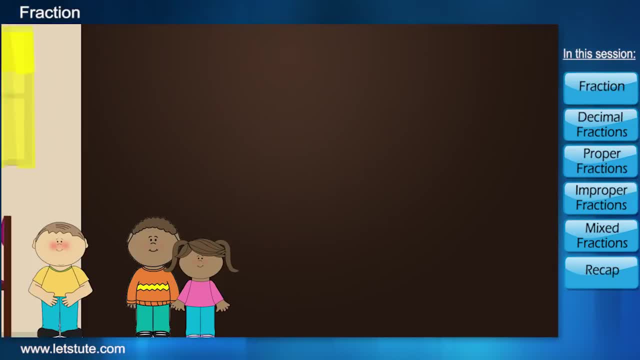 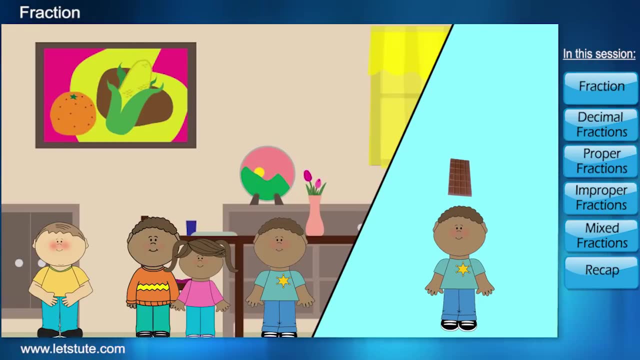 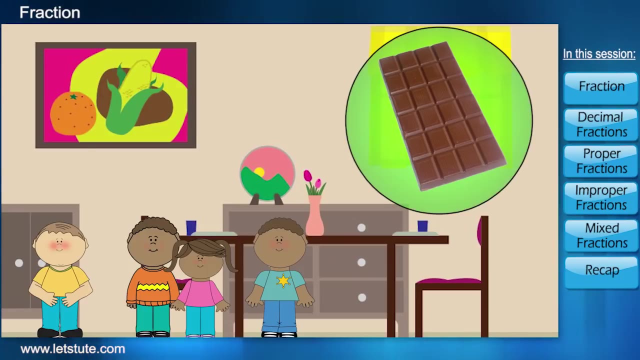 You and your two friends went to Ben's house. All the while waiting for you guys, he ate 9 out of the 10 chocolates that he kept for you guys. Now, after you guys reached, all you have is one big chocolate that you have to divide it in equal parts among your friends. 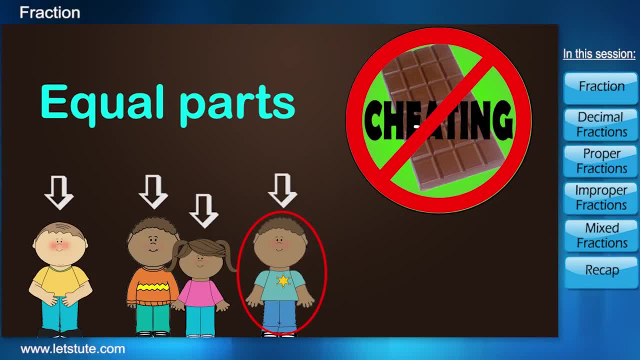 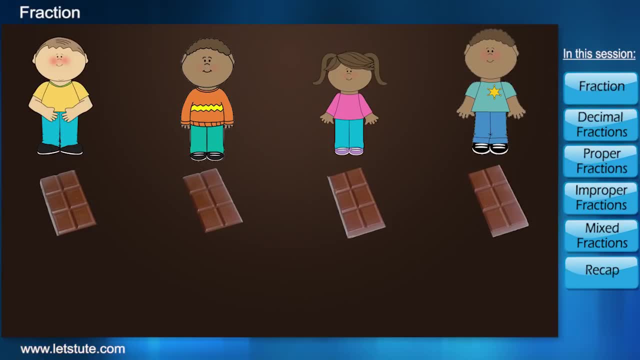 Including Ben No cheating. So how will you do that? Nice, You have divided one whole chocolate into four equal parts, So each one of you will get one part out of the four parts of the chocolate. Or can we say that each one of you had one fourth part of a chocolate? 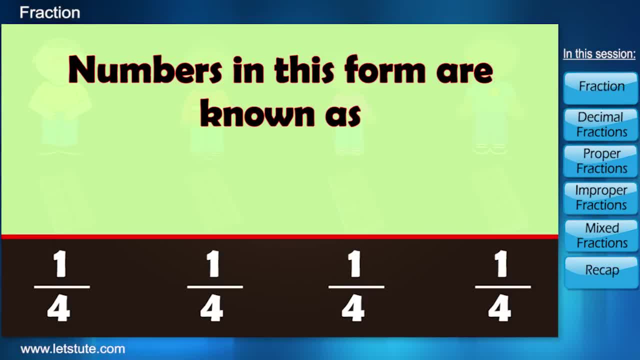 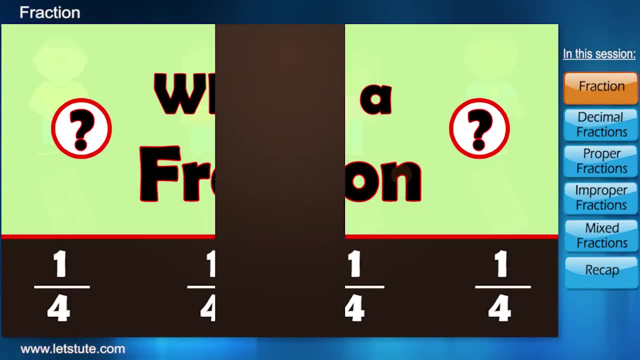 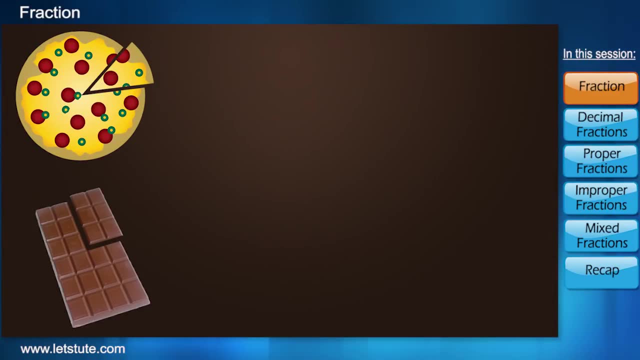 And numbers in this form are known as fractions. So what is a fraction? Fraction to a layman is just some part or a piece of something. The numbers of the form A by B are called fractions. Let's learn something more about fractions. 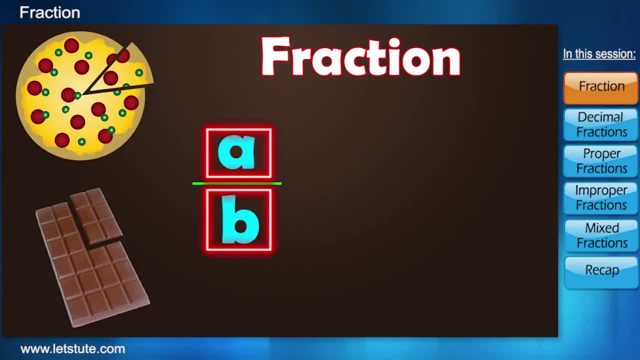 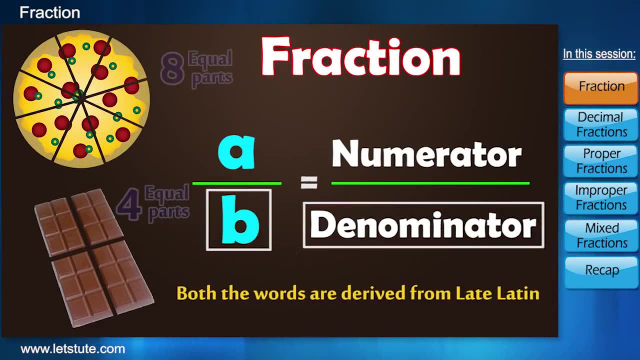 As we can see, a fraction has two parts: one top part and one bottom part. The top part is known as numerator and the bottom part is called as denominator. Denominator is the total number of equal parts in which the whole is divided into. 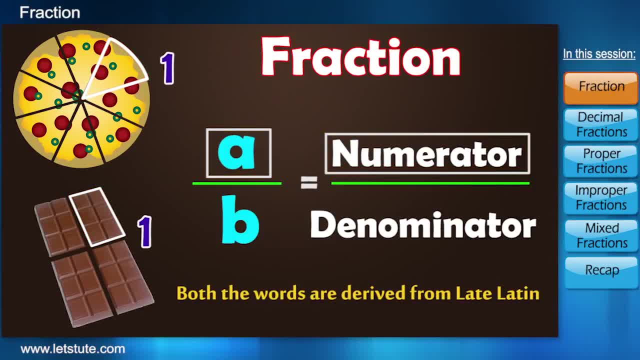 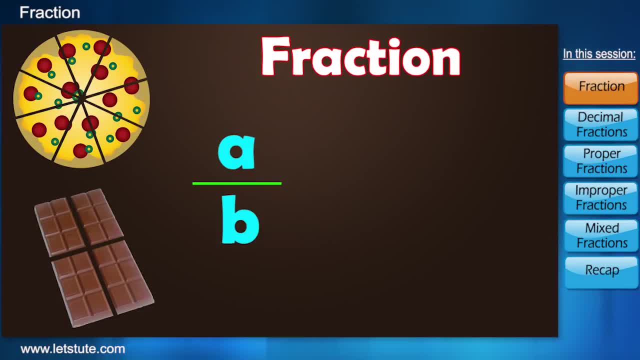 And numerator is the number of equal parts which have been taken out or which have been left out. Like as I said before, the numbers of the form A by B are called fractions, Where B cannot be zero. But why will it be zero? 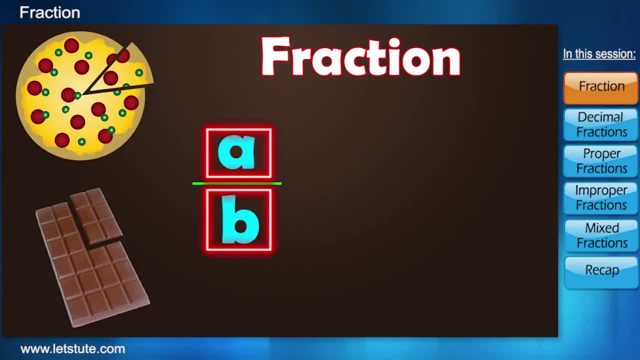 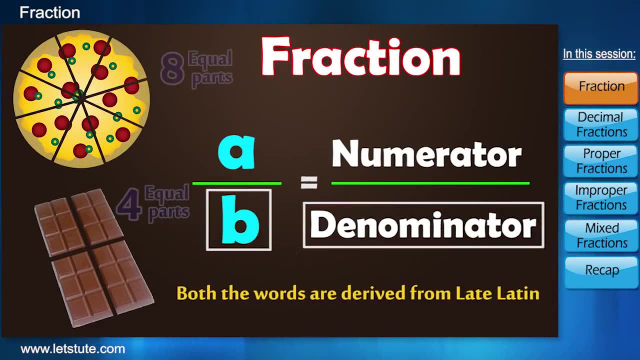 As we can see, a fraction has two parts: one top part and one bottom part. The top part is known as numerator and the bottom part is called as denominator. Denominator is the total number of equal parts in which the whole is divided into. 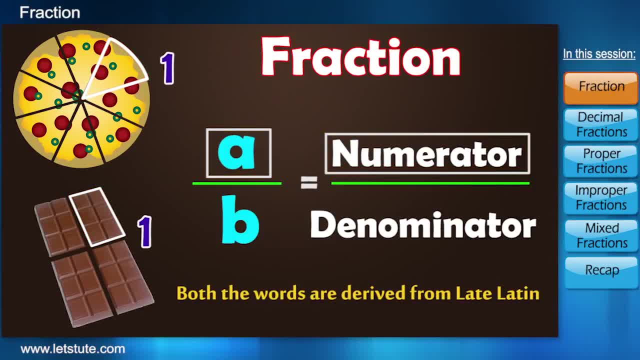 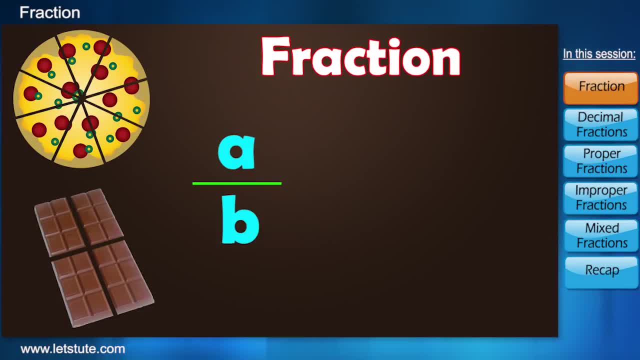 And numerator is the number of equal parts which have been taken out or which have been left out. Like as I said before, the numbers of the form A by B are called fractions, Where B cannot be zero. But why will it be zero? 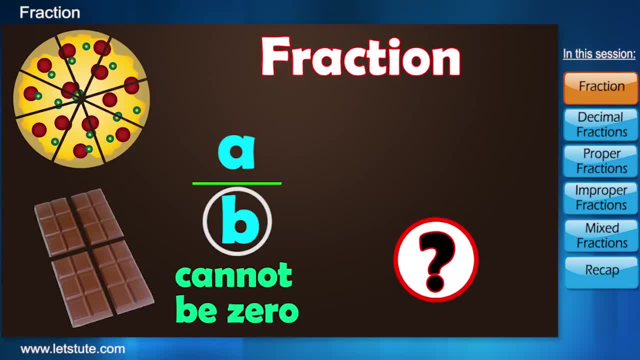 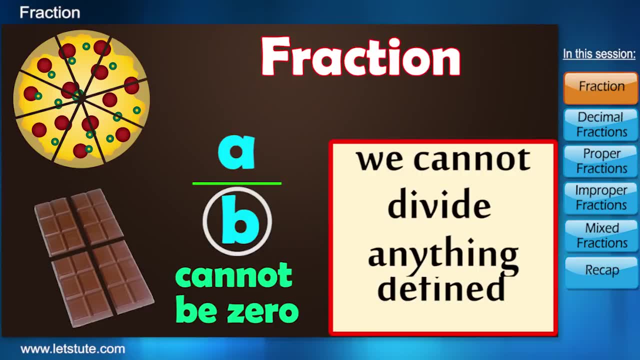 Because if it is zero, then the fraction will not be defined. Otherwise, we cannot divide anything by zero, As we cannot divide anything by zero confused. But why denominator cannot be zero? Basically, what is denominator? Denominator is the total number of equal parts. 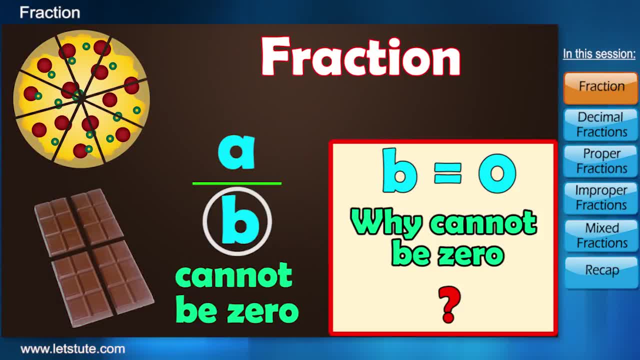 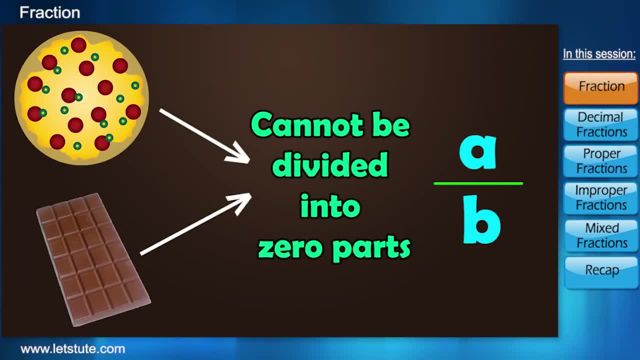 in which the whole is divided Right. But if we cannot divide anything by zero, divide anything into zero parts, we cannot give any part to anyone, and hence denominator of a fraction can never be zero. This is one of the golden rules of mathematics. 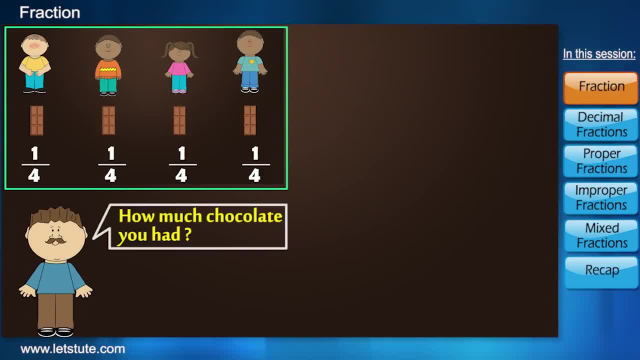 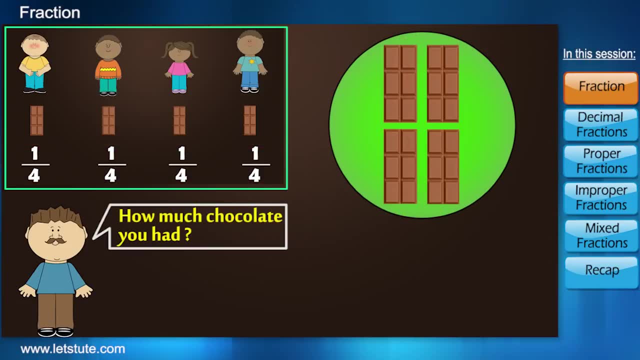 Now suppose your uncle asks you how much chocolate you had, You will not say you had one big chocolate. you divided it into four equal parts and ate one part of it. But now, as you know what fractions are, you will proudly say you ate one fourth part of the chocolate. 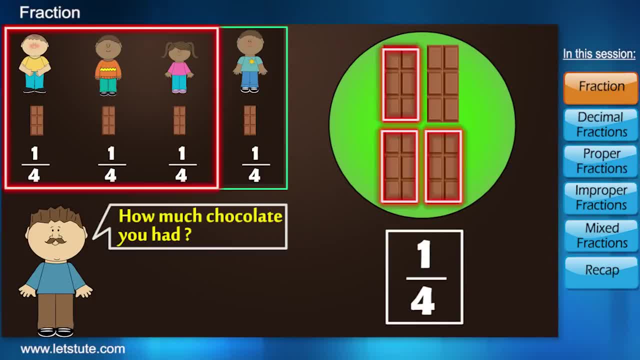 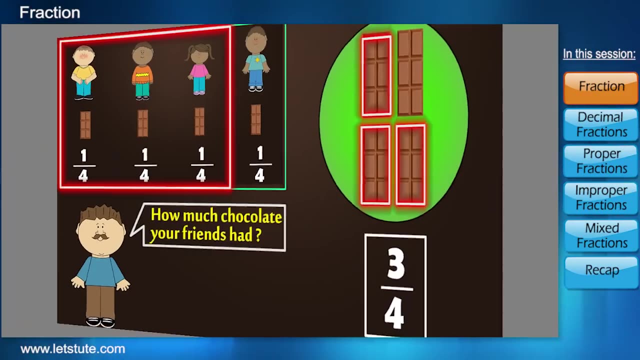 Now, can you tell me how much part of the chocolate did all your remaining friends have? Three parts of the chocolate were remaining out of four, So they all had three fourth part of the chocolate. Let's take a small quiz before we move ahead. Can you tell me that do the shaded region? 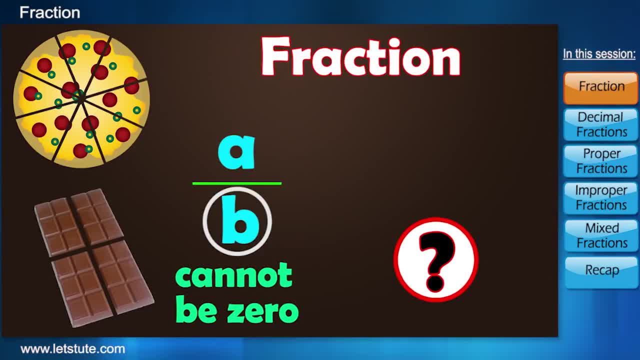 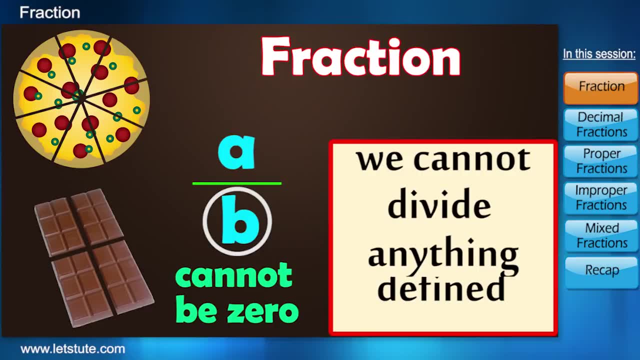 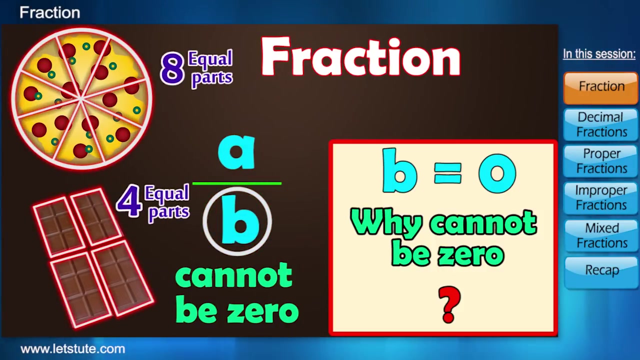 Because if it is zero, then the fraction will not be defined, As we cannot divide anything by zero. Confused. But why denominator cannot be zero? Basically, what is denominator? Denominator is the total number of equal parts in which the whole is divided. 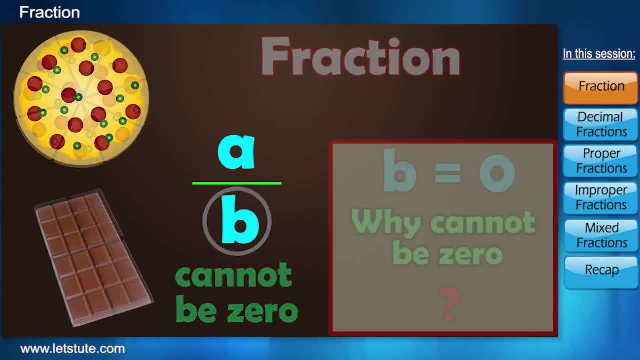 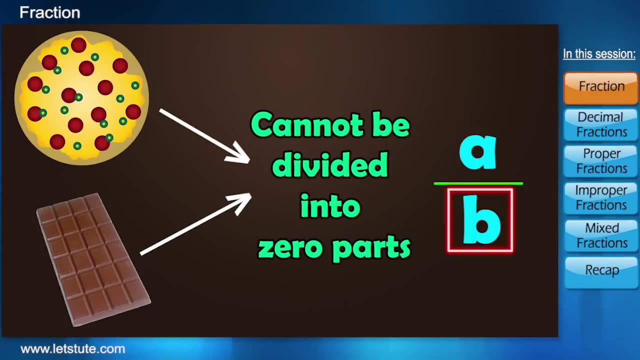 Right, But if we cannot divide anything by zero, then why can't we divide by zero? We cannot give any part to anyone, And hence denominator of a fraction can never be zero. This is one of the golden rules of mathematics. Now suppose your uncle asks you how much chocolate you had. 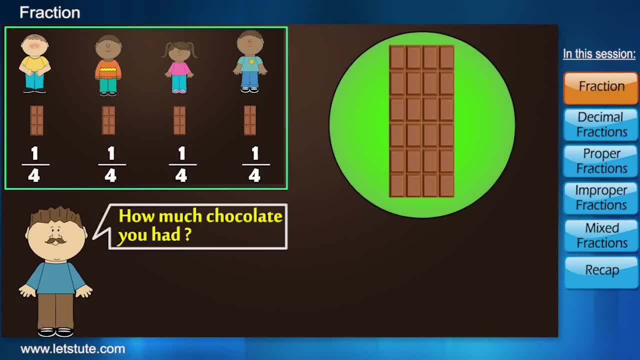 You will not say: you had one big chocolate. you divided it into four equal parts and ate one part of it. But now, as you know what fractions are, you will proudly say you ate one fourth part of the chocolate. Now can you tell me how much part of the chocolate did all your remaining friends have? 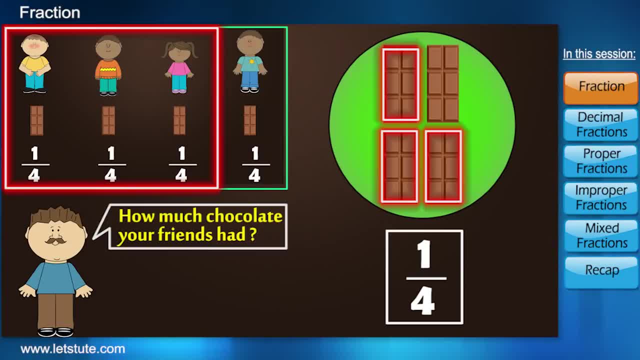 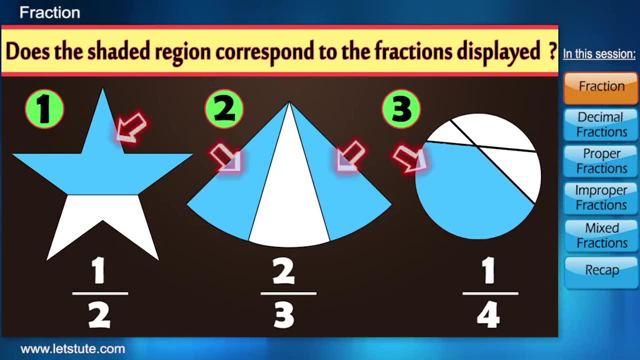 Three parts of the chocolate were remaining out of four, So they all had three fourth part of the chocolate. Let's take a small quiz before we move ahead. Can you tell me that? do the shaded region correspond the fractions displayed In question 2,? the shaded region represents the fraction, but not in the other two. 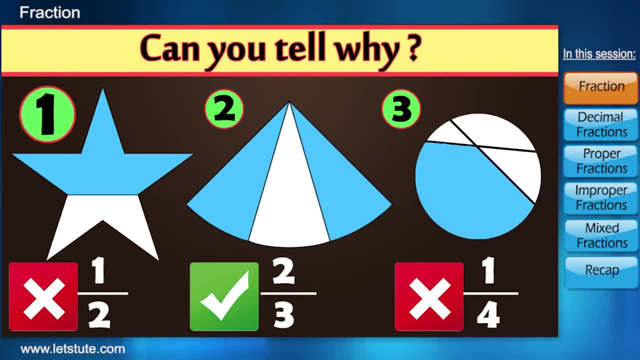 Can you tell why In figure 1, it is not divided into two equal parts And in figure 3, it is not divided into four equal parts And hence the fractions are not corresponding the shaded regions? Did you get all the three correct? 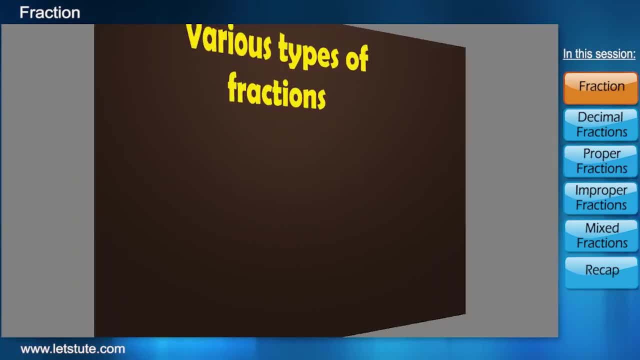 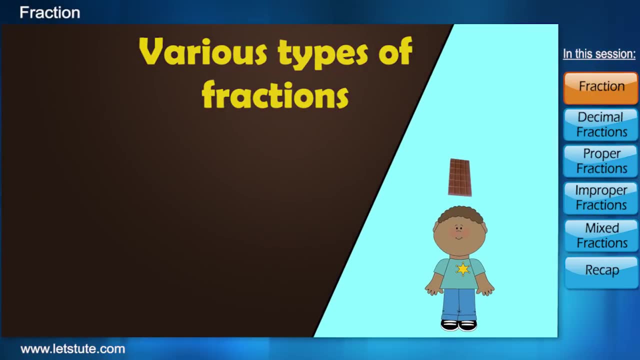 Let's take a step further, learning the various types of fractions. As you guys were late, Ben ate nine out of the ten chocolates. Imagine if Ben had hundred or thousand or ten thousand chocolates. Imagine if Ben had hundred or thousand or ten thousand chocolates. 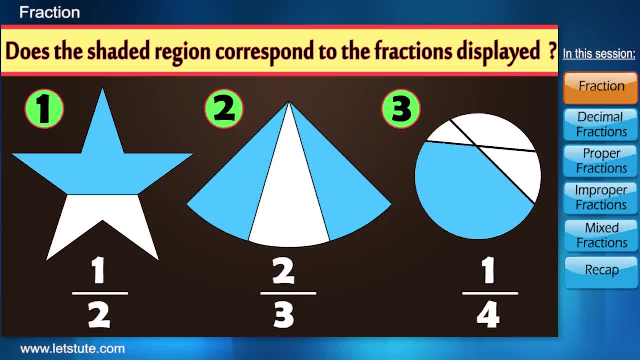 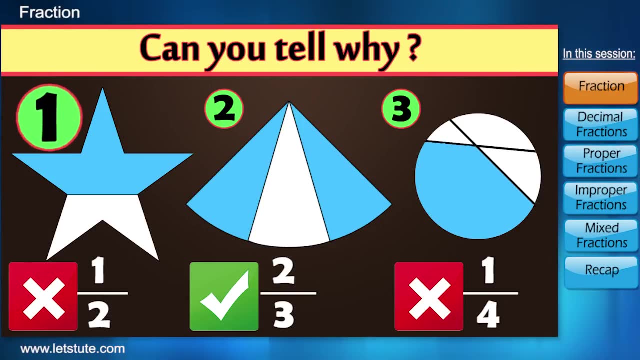 correspond the fractions displayed. In question 2, the shaded region represents the fraction, but not in the other two. Can you tell why In figure 1, it is not divided into two equal parts and in figure 3, it is not divided into four equal parts and hence the fraction? 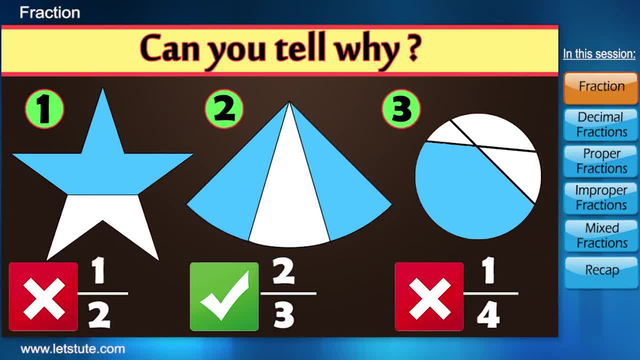 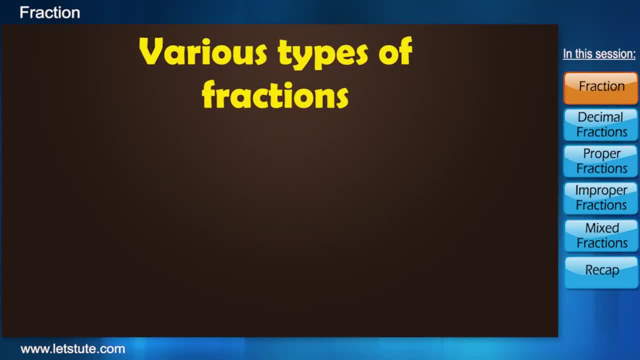 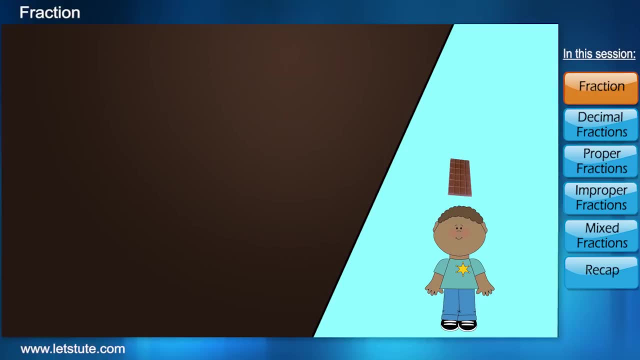 are not corresponding the shaded regions. Did you get all the three correct? Let's take a step further, learning the various types of fractions. As you guys were late, Ben ate nine out of the ten chocolates. Imagine if Ben had 100 chocolates. Can you tell me how? 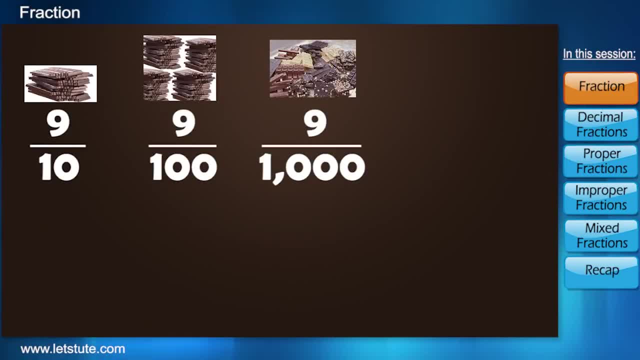 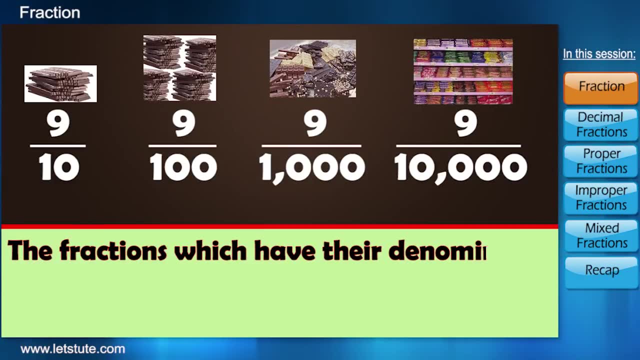 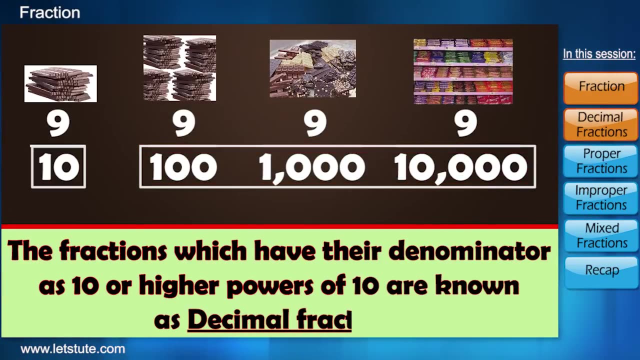 many can a person eat? And how can a person eat, Whether they are hundreds of 1000's or 1000's or 10,000 chocolates? So here, the fractions which have the denominator as 10 or higher powers of 10 are known as decimal fractions. 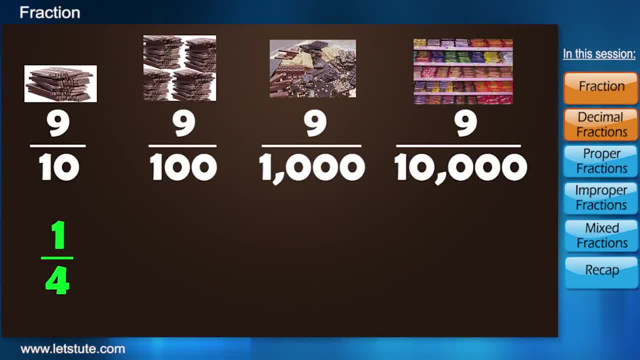 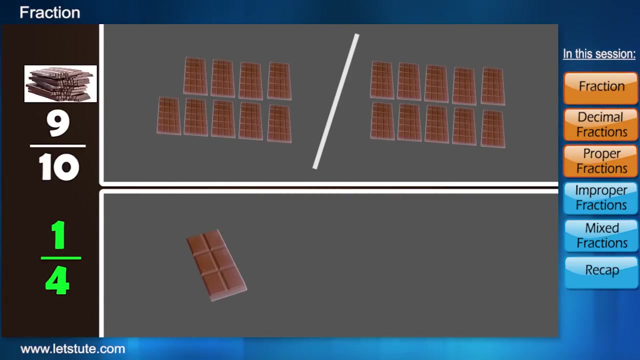 Till now. whichever examples we saw, all these are proper fractions. Proper fractions are the fractions where the number of fractions does not matter. For instance, when we add, the numerator is smaller than the denominator. Taking out nine chocolates from a pack of ten chocolates or taking one piece from a chocolate which is divided into four equal. 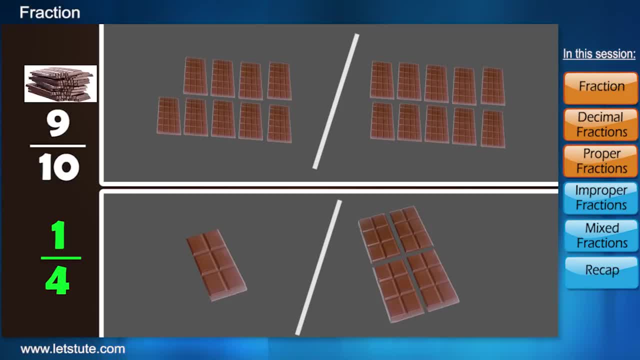 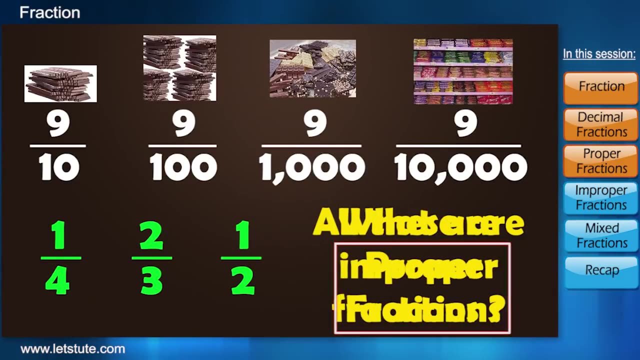 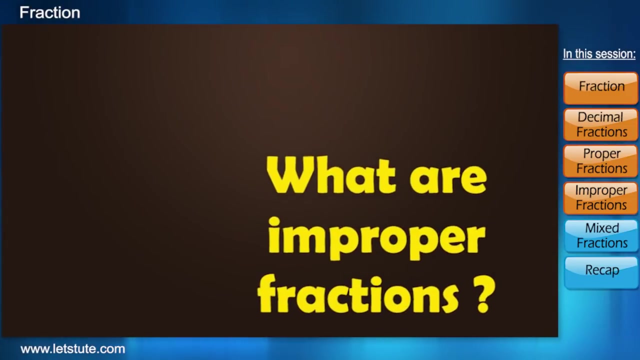 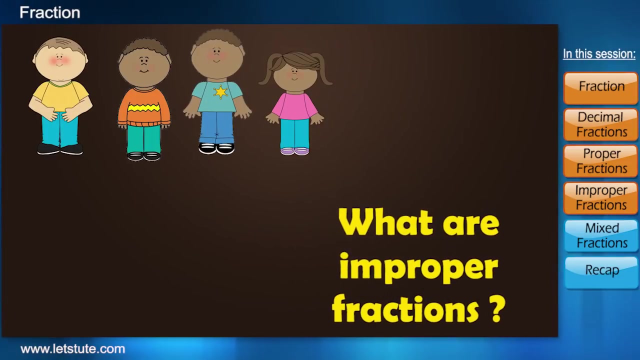 pieces. These examples will make only proper fractions because their numerator is always smaller than the denominator. If all the fractions that we have studied till now are proper fractions, then what are improper fractions? Nothing is basically improper with these fractions. These are just called as improper fractions. If you guys had five chocolates instead of 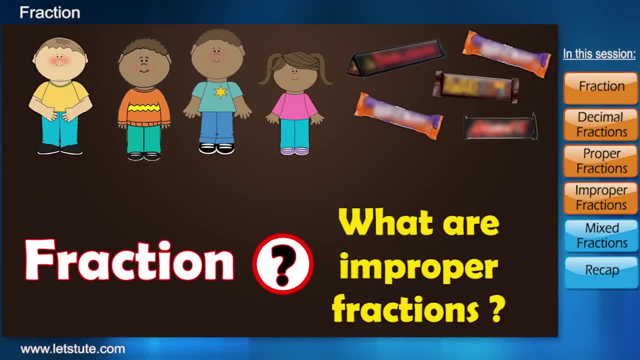 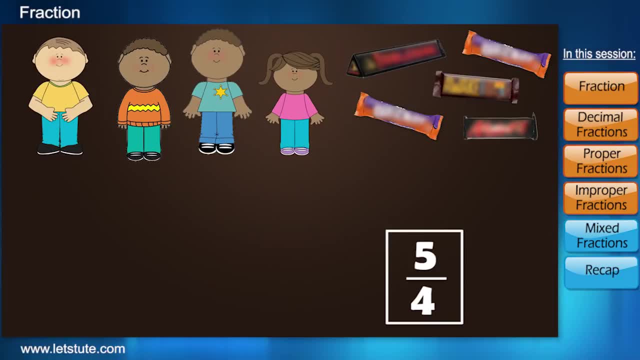 one, then what will be the fraction formed? The fraction formed is 5 divided by 4, and this is an improper fraction. Improper fractions are the fractions where the numerator is bigger than the denominator, Like 10 by 9 or 6 by. 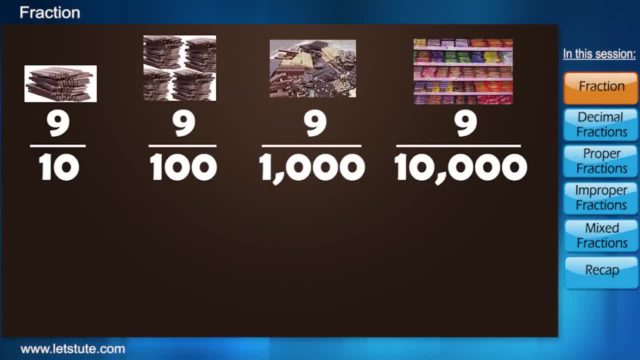 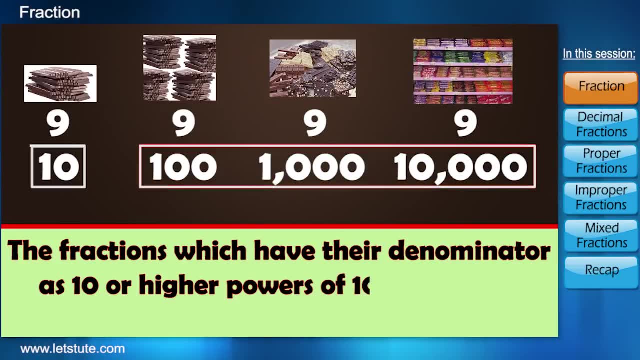 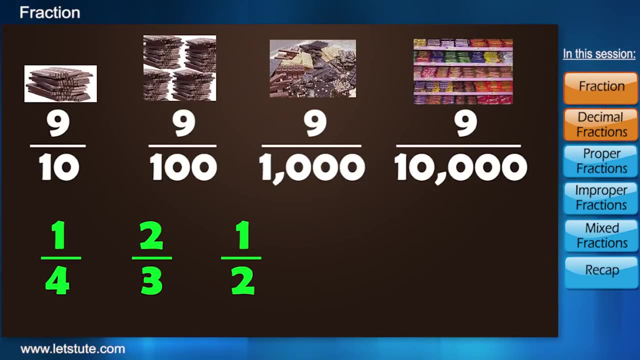 Imagine if Ben had hundred or thousand chocolates. So here, the fractions which have the denominator as ten or higher powers of ten are known as decimal fractions. Till now, whichever examples we saw, all these are proper fractions. Proper fractions are the fractions where the numerator is smaller than the denominator. 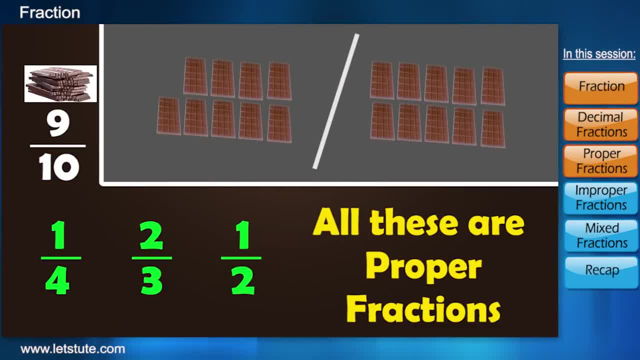 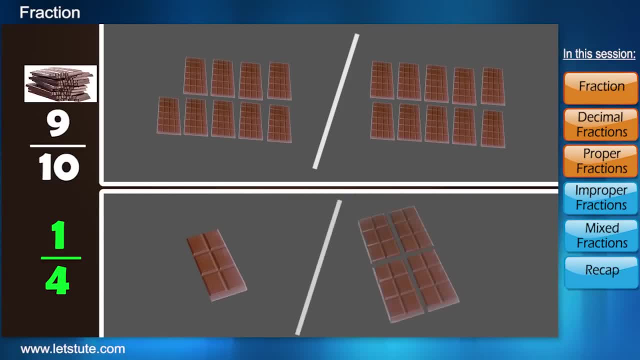 Proper fractions are the fractions where the numerator is smaller than the denominator. Taking out nine chocolates from a pack of ten chocolates. Taking out nine chocolates from a pack of ten chocolates, Or taking one piece from a chocolate which is divided into four equal pieces. 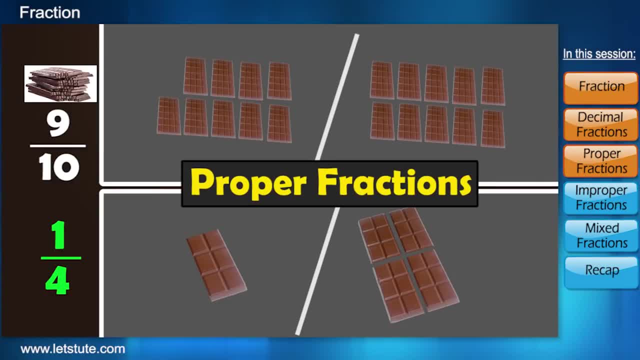 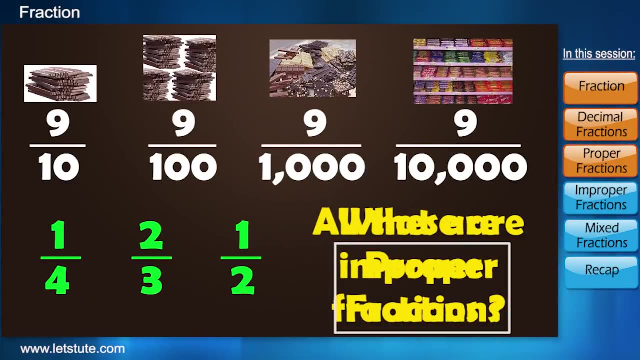 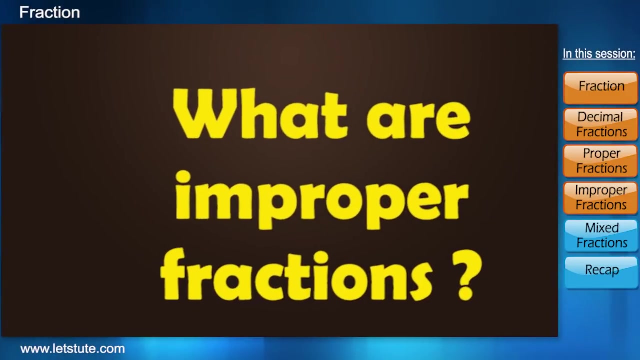 These examples will make only proper fractions because their numerator is always smaller than the denominator. If all the fractions that we have studied till now are proper fractions, If all the fractions that we have studied till now are proper fractions, what are improper fractions? Nothing is basically improper with these fractions. 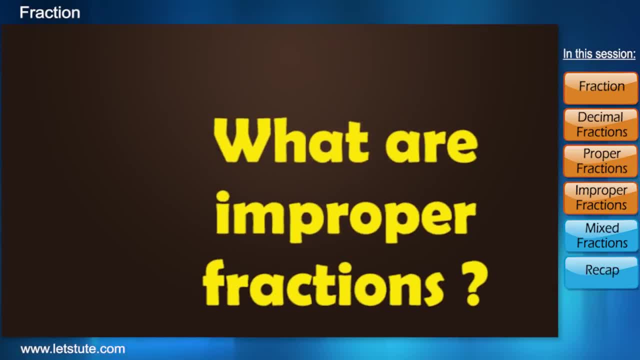 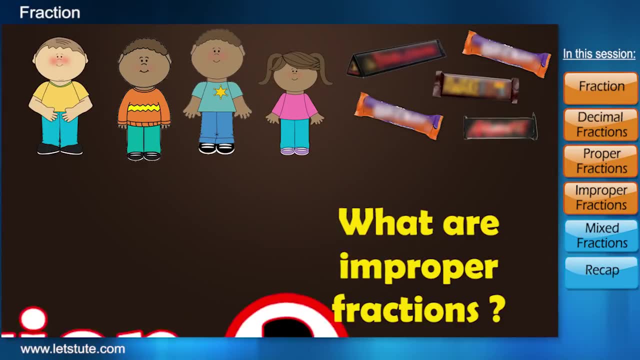 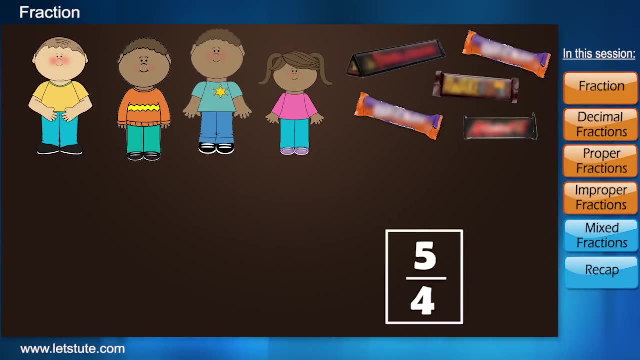 These are just called as improper fractions. If you guys had five chocolates instead of one, If you guys had five chocolates instead of one, then what will be the fraction formed? The fraction formed is five divided by four, And this is an improper fraction. 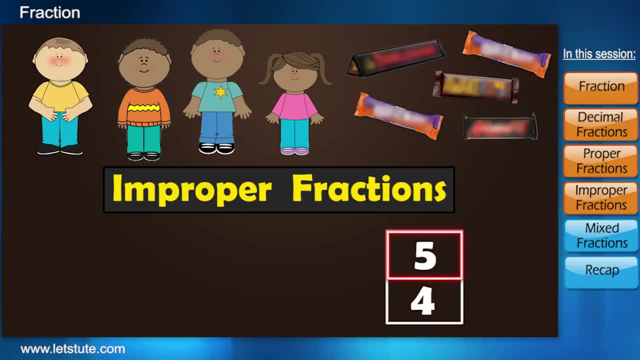 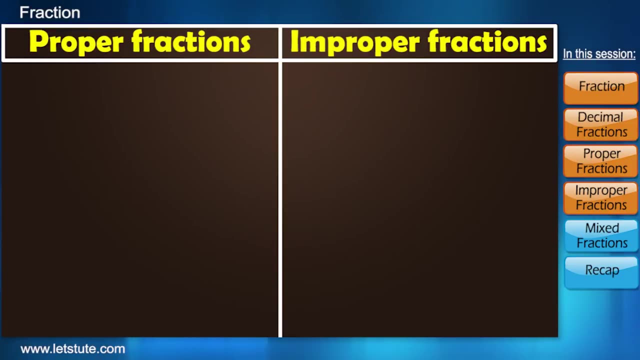 Improper fractions are the fractions where the numerator is bigger than the denominator, Like ten by nine or six by five. Do not confuse yourself between proper and improper fractions. Whenever we perform a normal division on a proper fraction, the answer will always be less than one. 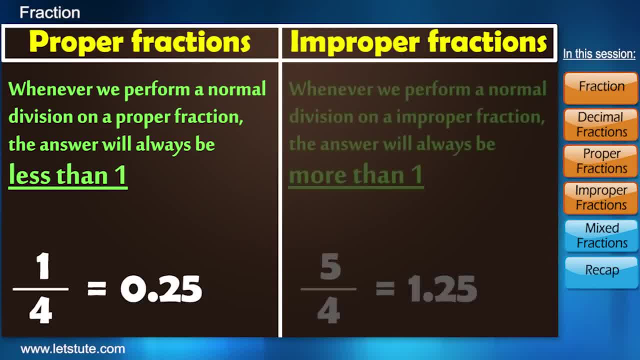 And with improper fractions, there will always be more than one. Less than one is proper and more than one is improper. Are we good till here? Let's move on. Improper fractions can be further written in a different manner. We just saw an example of improper fractions. 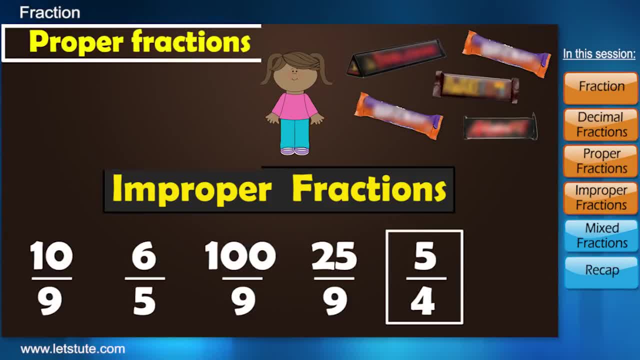 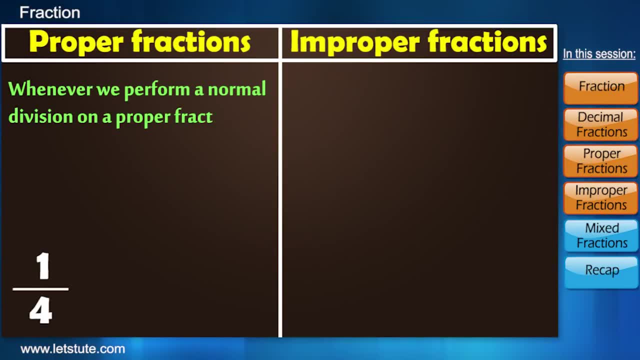 5. Do not confuse yourself between proper and improper fractions. Whenever we perform a normal division on a proper fraction, we have to be careful not to confuse ourselves with improper fractions. Whenever we perform a normal division on a proper fraction, we have to be careful not to confuse ourselves with improper fractions Whenever we perform. 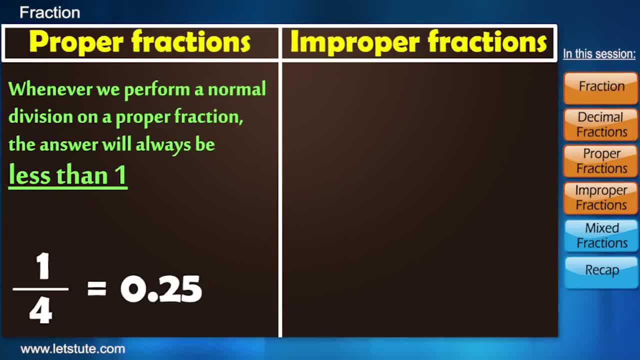 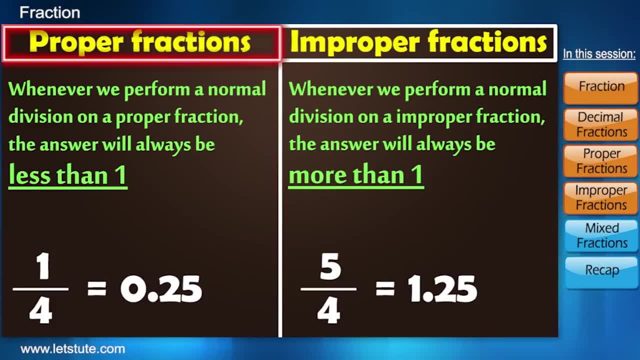 a normal division on a proper fraction, we have to be careful not to confuse ourselves with improper fractions. The answer will always be less than 1 and with improper fractions it will always be more than 1.. Less than 1 is proper and more than 1 is improper. Are we good till? 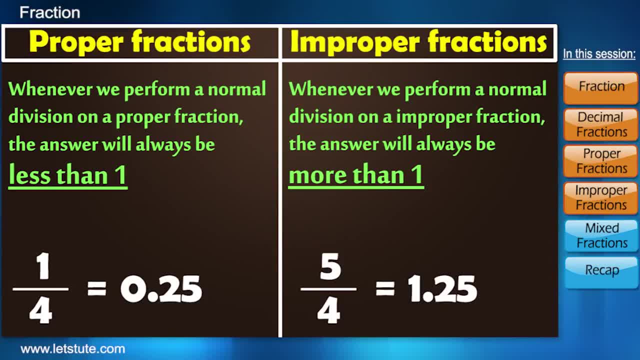 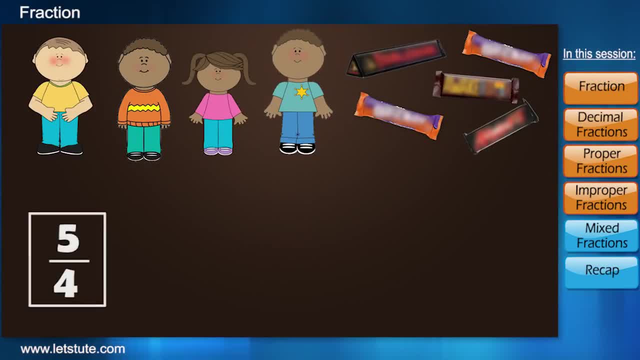 here, Let's move on. Improper fractions can be further written in a different manner. We just saw an example of improper fractions: 5 divided by 4.. You guys have to be careful not to confuse yourselves with improper fractions. You guys had 5 chocolates and only 4 friends. Now how will you divide? 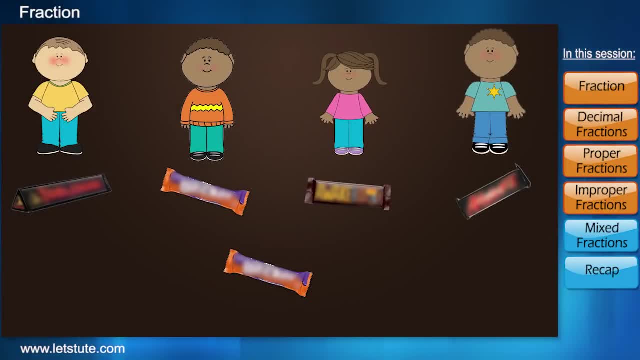 this among yourselves. You guys can take 1 chocolate each at first. Now you are left with one chocolate and 4 people. Same problem with which we started this session Right. So we know each one of you will get one-fourth part of the chocolate. So now we are done. 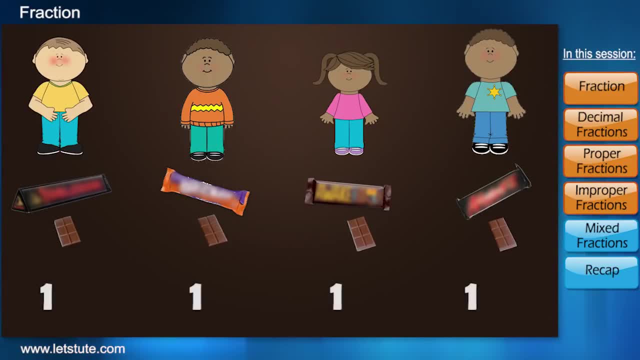 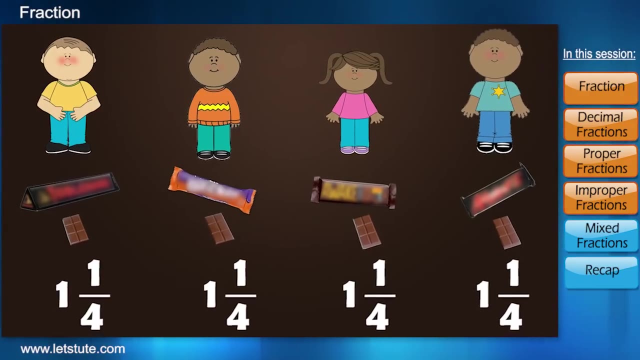 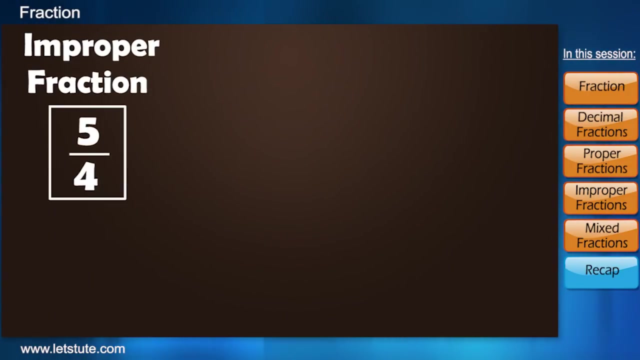 Now each one of you guys have one chocolate and one-fourth part of the other chocolate. In total, you have one one-fourth chocolate, right? All these fractions are known as mixed fractions. You can also obtain mixed fraction by performing a normal division. 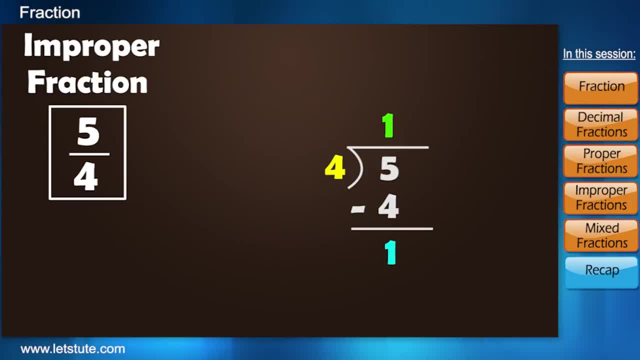 Let's see how we can do that. A mixed fraction is written as quotient remainder, divided by divisor. So here it will be one, one by four, right, Because one is the quotient, one is also a remainder and four is the divisor. 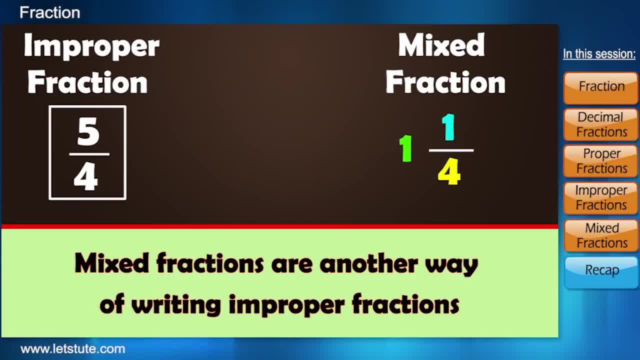 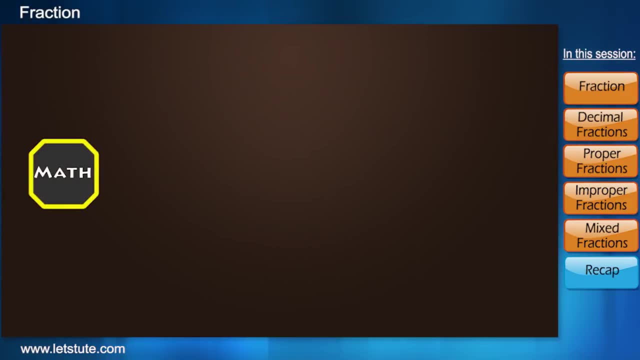 Mixed fractions are written as quotient remainder divided by divisor. These are nothing but another way of writing improper fractions. In this process, we have also learnt how to convert an improper fraction into a mixed fraction. Isn't this amazing when you understand one thing and you can apply them at many places? 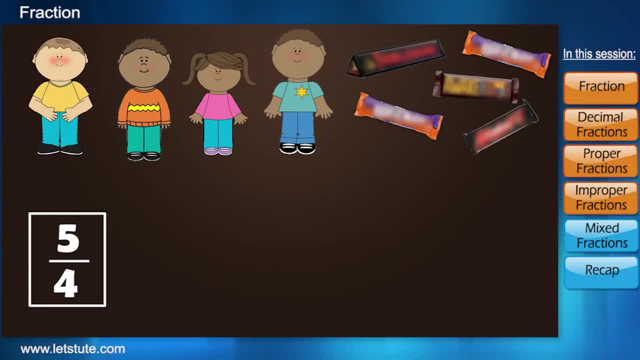 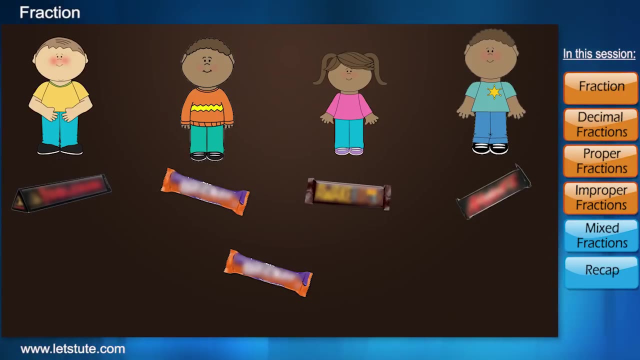 Five divided by four. You guys had five chocolates and only four friends. Now how will you guys divide this among yourselves? You guys can take one chocolate each at first. Now you are left with one chocolate and four people. Same problem with which we started this session. 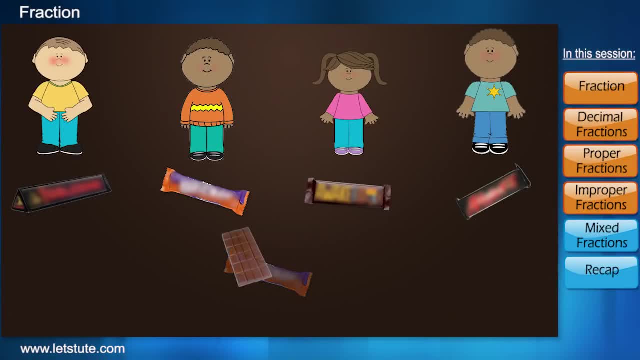 Right. So we know each one of you will get one fourth part of the chocolate. So now each one of you guys have one chocolate and one fourth part of the other chocolate. In total, you have one one fourth chocolate, Right. 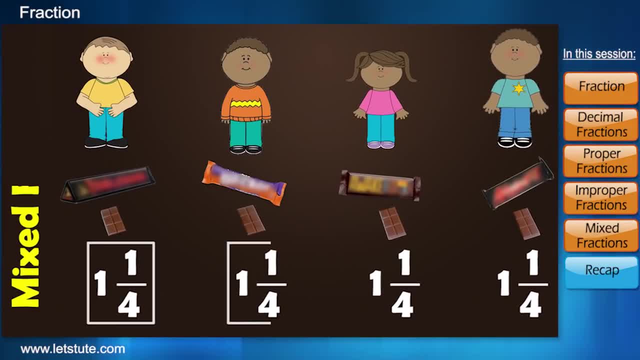 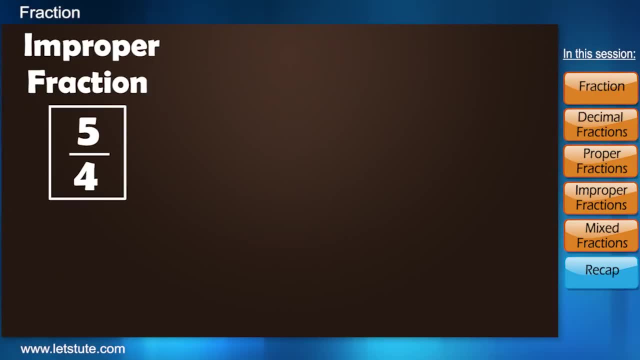 All these fractions are known as mixed fractions. You can also obtain mixed fraction by performing a normal division. Let's see how we can do that. A mixed fraction is written as. A mixed fraction is written as question remainder divided by divisor. So here: 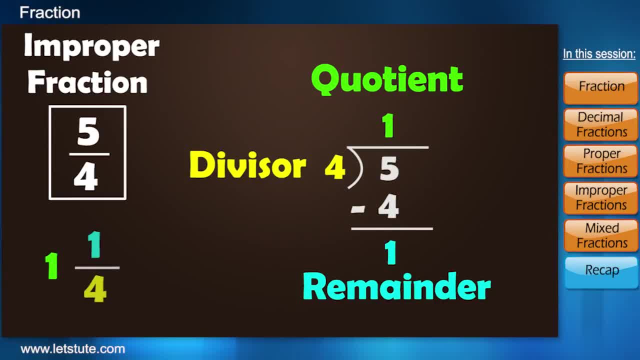 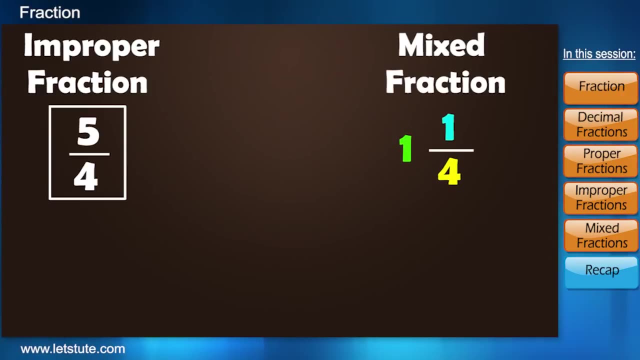 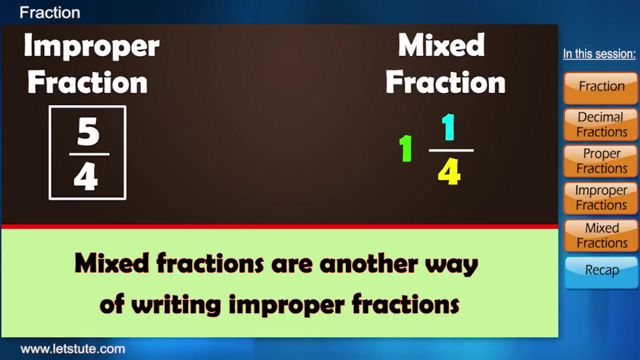 it will be one, one by four. Right, Because one is the question, one is also a remainder and four is the divisor. Mixed fractions are nothing but another way of writing improper fractions. In this process, we have also learnt how to convert an improper fraction into a mixed fraction. 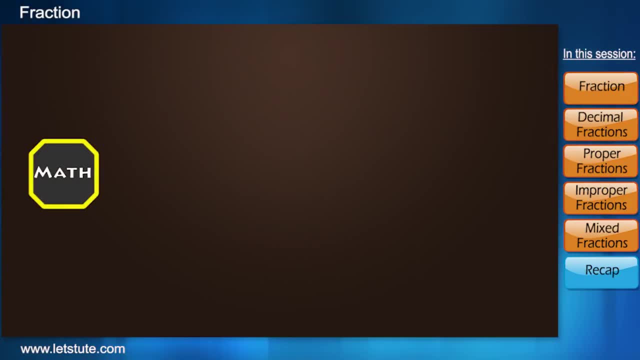 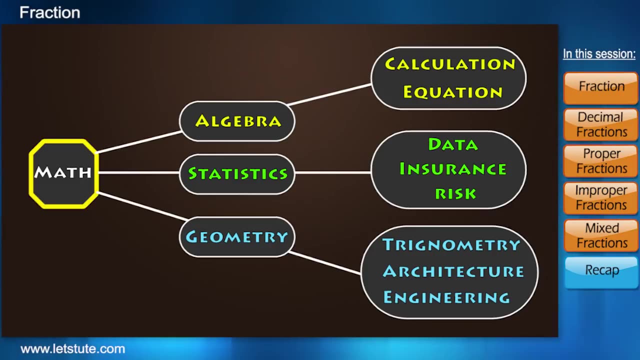 Isn't this amazing: when you understand one thing and you can apply them at many places. This is just another beauty of understanding things rather than mugging them up. So let's have a recap before we finish this session. What are fractions? 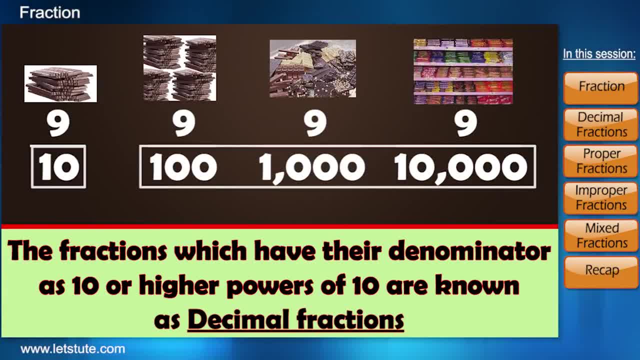 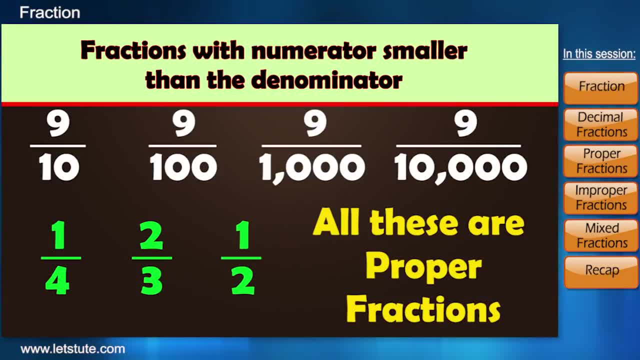 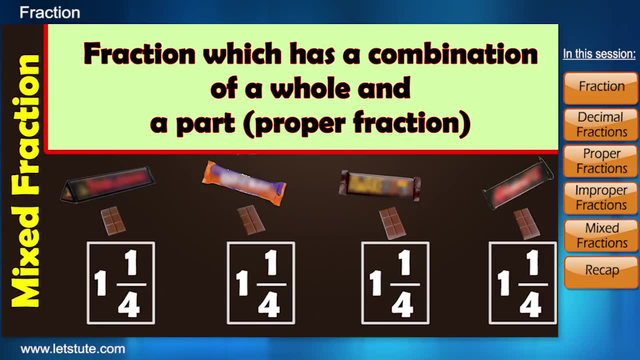 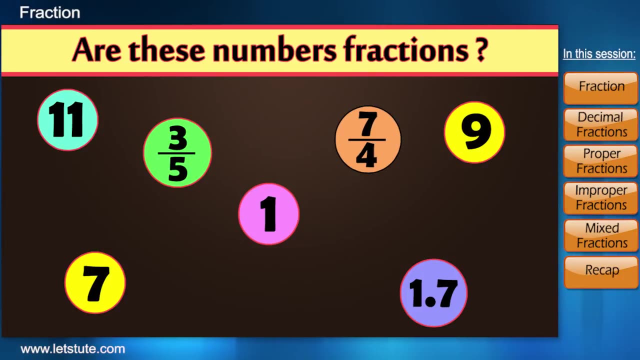 and four types of them. Before I leave, can you tell me that? are these numbers also fractions? I'll be excited to know your answers and you can put them in the comments below. And do hit the like button In our next session.